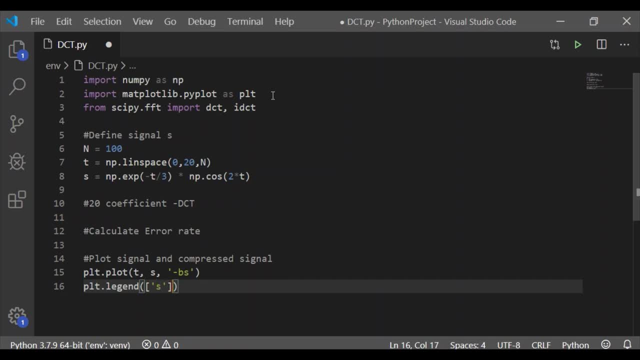 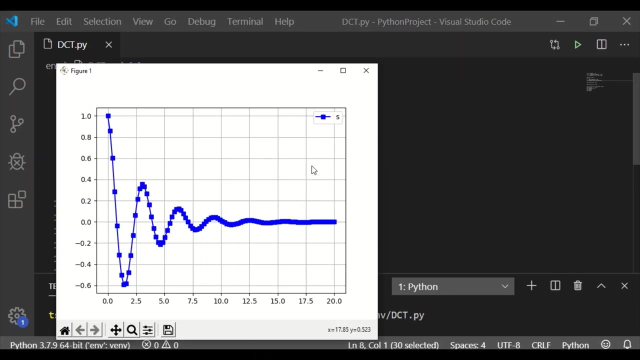 of exponential minus t by 3, multiplied by cos 2t. let us give the legend yes on the plot, because in the same plot, sooner, we will be plotting the reconstructed signal or the compressed signal. so now let me execute it to visualize the original signal. we could see our original signal. yes is. 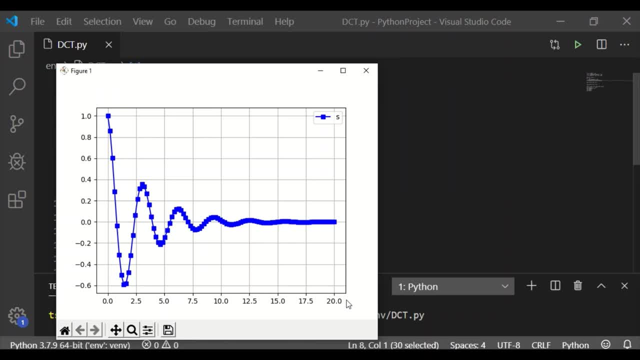 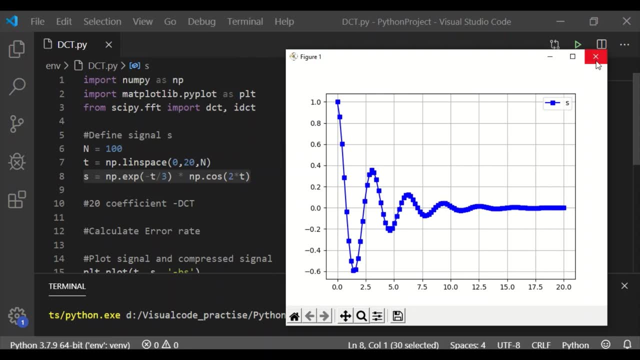 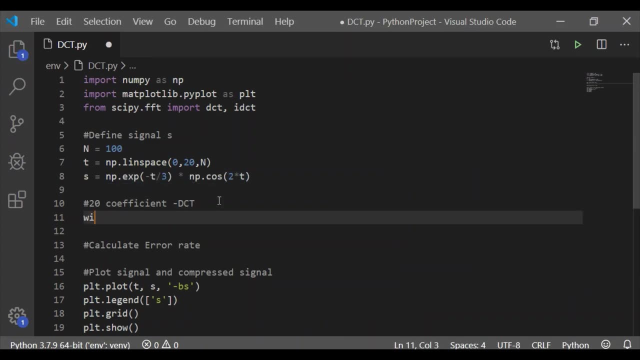 plotted along the t values of 0 to 20, and it has 100 unique values. now coming to the second step, we are going to reconstruct the signal by using only 20 coefficients of discrete cosine transform on the original signal. so we will have the list windows. 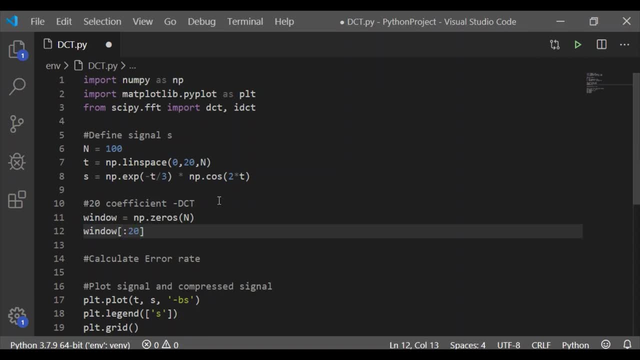 which has 100 elements, out of which first 20 is initialized to 1 and 21 to 100, takes the value of 0. in order to get the coefficients of dct first, we will do the discrete cosine transform on our original signal. yes, using dct. yes, and we will do it as a normalized dct. and yr is the. 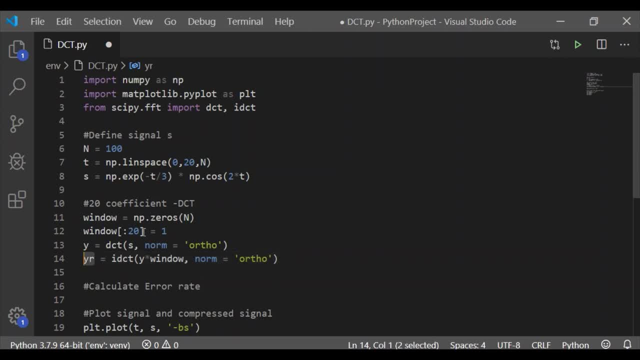 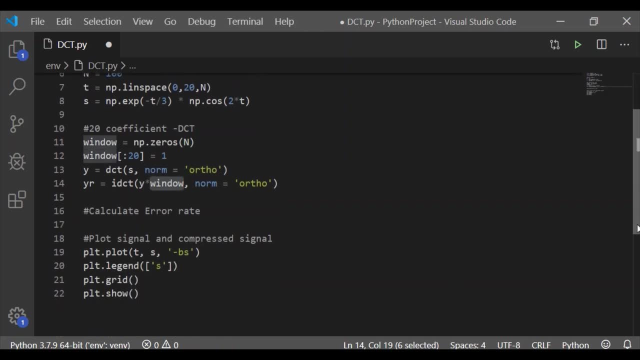 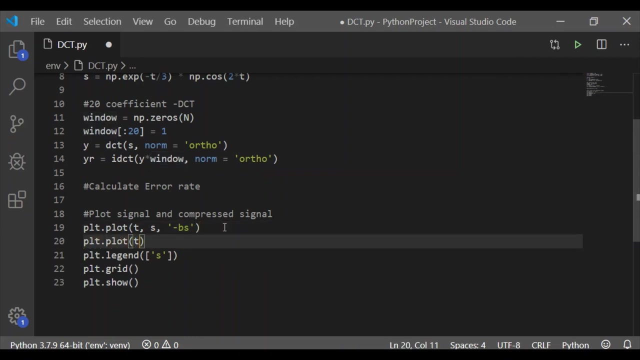 instrumented inverse DCT by having only 20 coefficients, so Y, the DCT multiplied by window, which has one for only first 20 elements. so YR is the inverse normalized DCT signal. as in step 1, we have plotted our original signal. now again, at the end of step 2, we are moving to 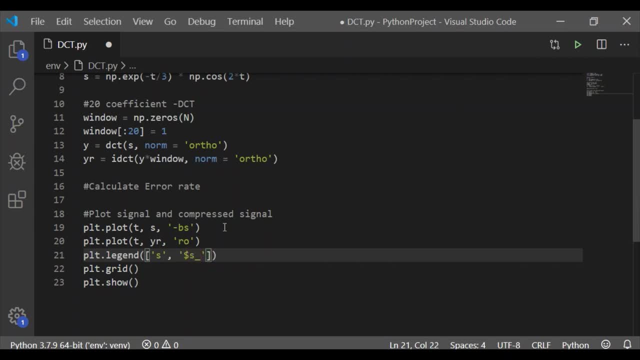 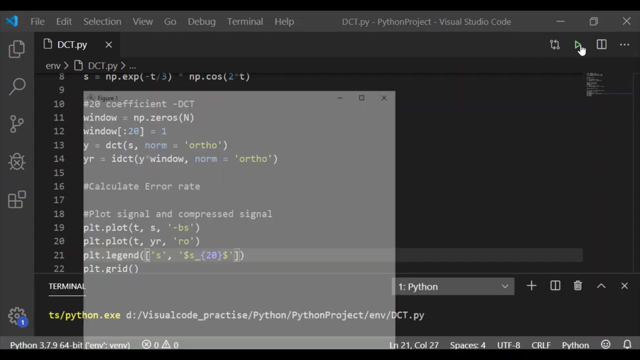 plot our reconstructed signal using 20 coefficient of DCT, that is, YR. it shall be red color with marker O filled in marker of O. so on executing, we could see that both the original signal- yes, with 100% of the original signal- we have plotted our original signal. now again at the